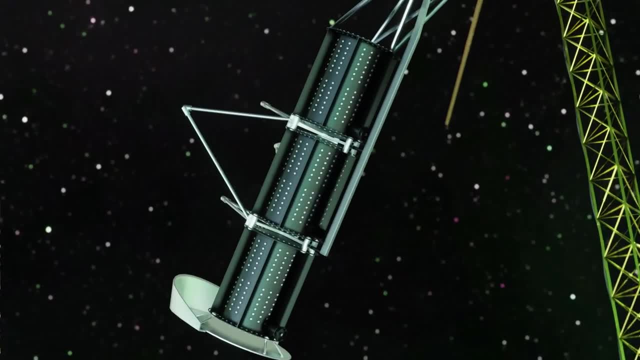 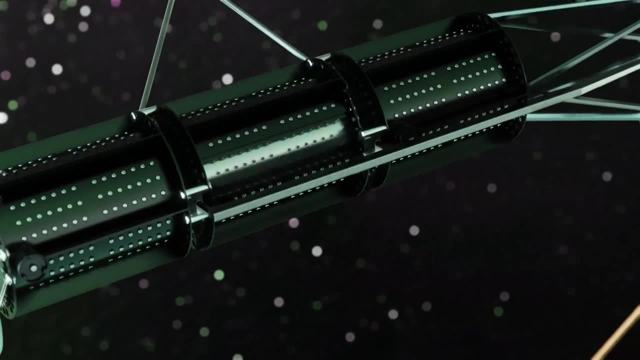 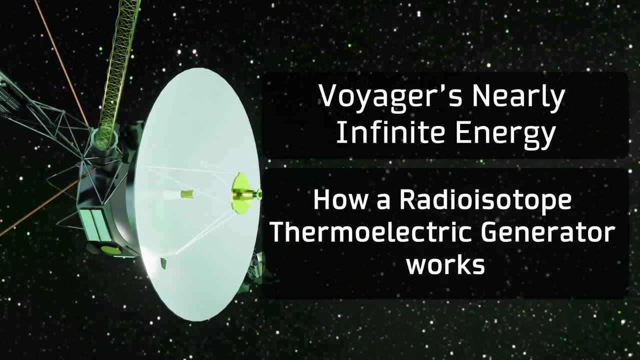 it to operate. What's more, according to NASA itself, to this day, none of these generators, also used on other missions, have ever stopped producing electricity, And that is why, in this video, we will talk about Voyager's almost infinite unexpected power, or, more specifically, how a radioisotope thermoelectric generator 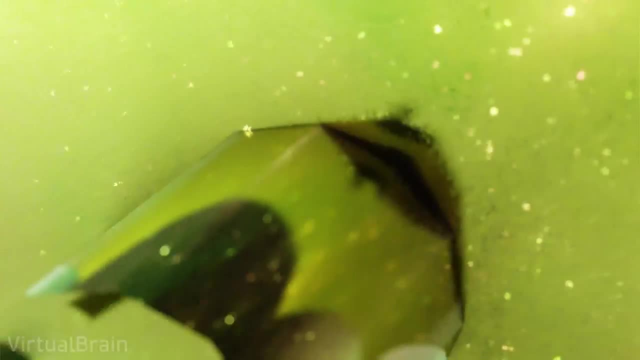 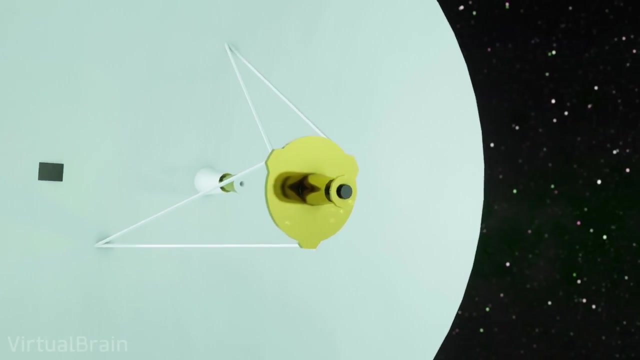 also known as nuclear batteries, can do it. Let's start with a bit of context before getting into the technical part, Although the Voyager probes are not the only ones that use this type of generators. Voyager 1 is currently the farthest man-made object from planet Earth. 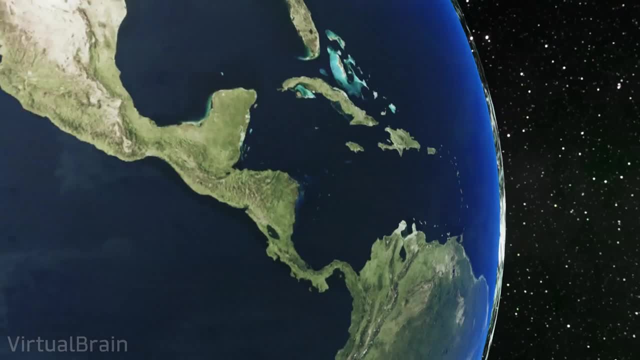 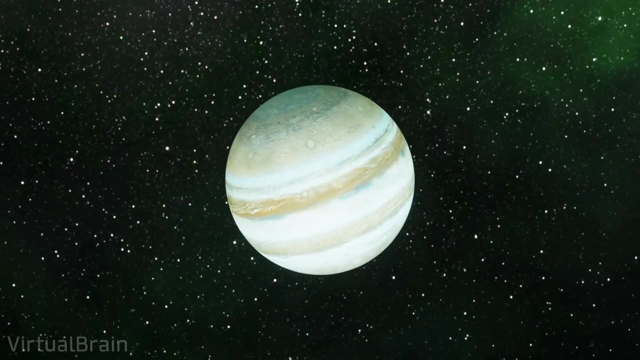 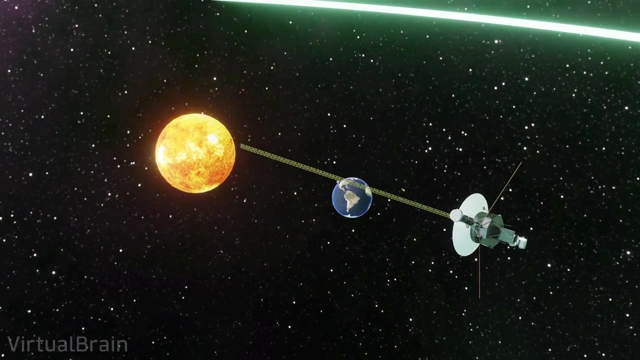 So I thought it was a good opportunity to talk about them. space probes were launched in 1977 with the main goal of exploring Jupiter and Saturn, along with other planets of the solar system. The mission was initially projected to last five years, but to this day both probes continue. 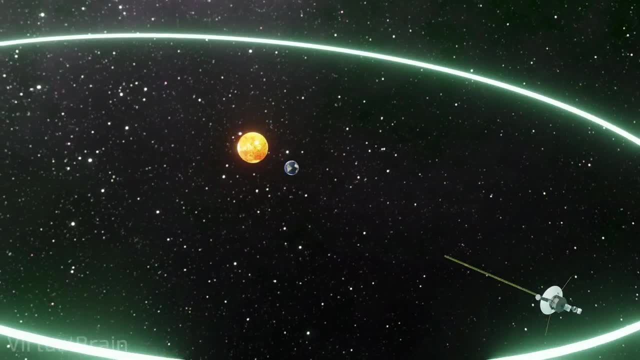 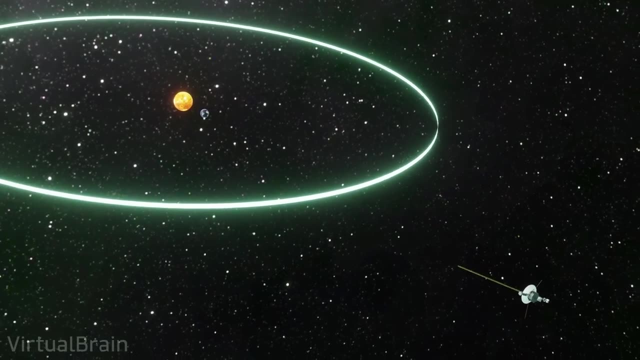 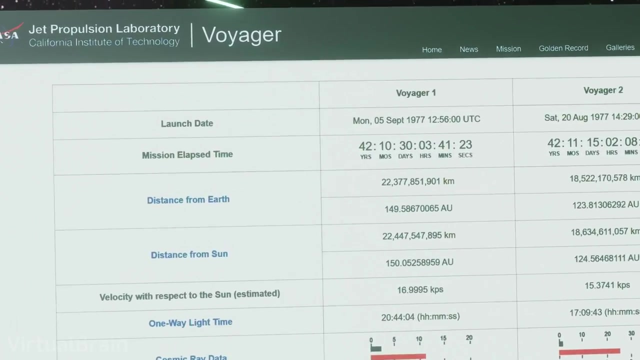 to send data from beyond the Aleopause, which they crossed in 2012, and which corresponds to the theoretical limit where the influence of the solar system ends and interstellar space begins. At the time of this animation, the Voyager 1 probe is 22 billion kilometers from planet. 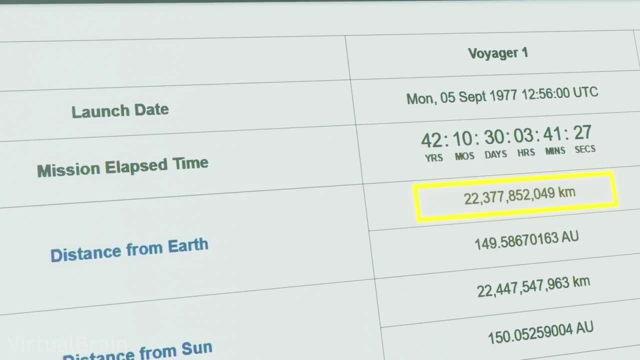 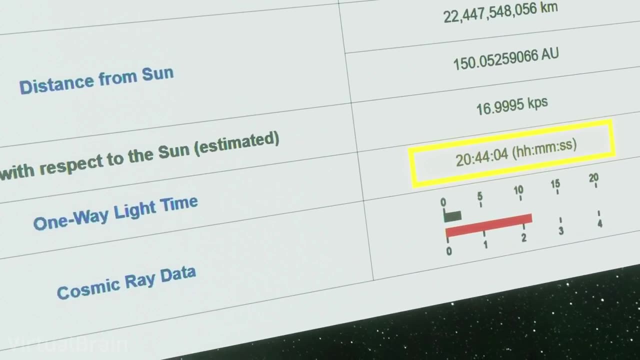 Earth, a distance so unimaginably great that the signals sent, which travel at the speed of light, take more than 20 hours to reach the Earth. To give you a point of reference, sunlight takes, on average, about 8 minutes and 20 seconds. 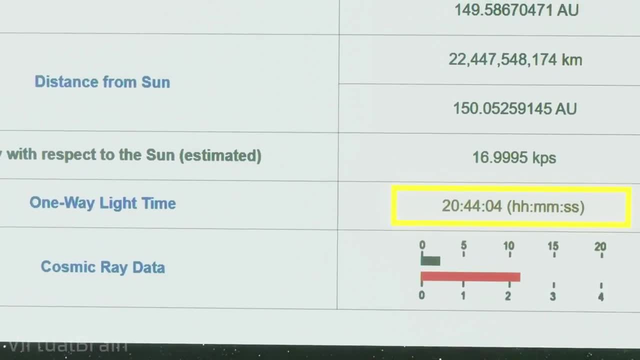 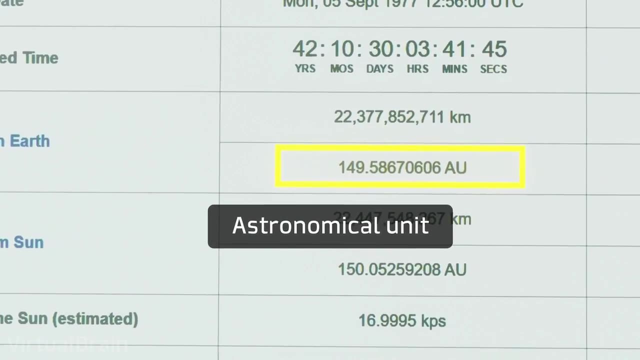 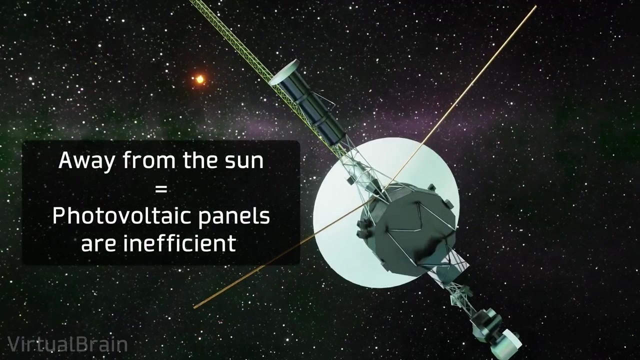 to reach the Earth. In other words, the Voyager 1 probe is located 149 times the distance between the Earth and the Sun, a unit known as an astronomical unit. At such a great distance from the Sun, the amount of light the probes receive is so small. 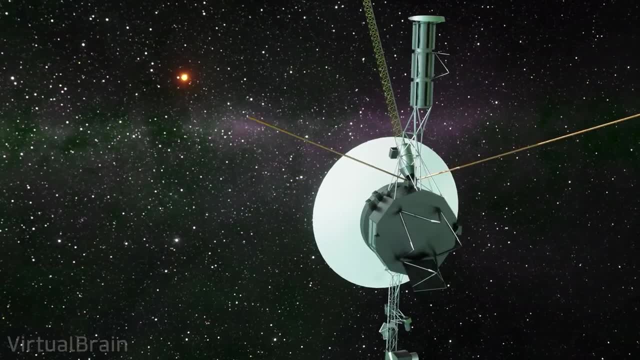 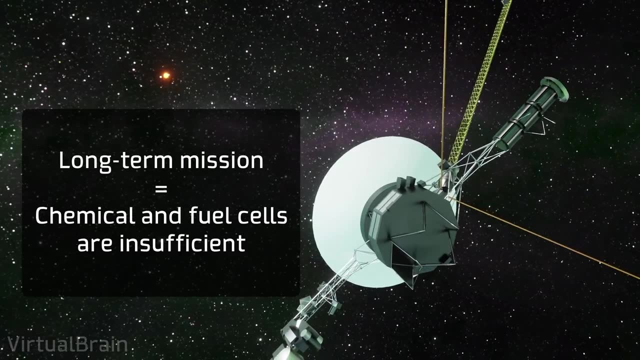 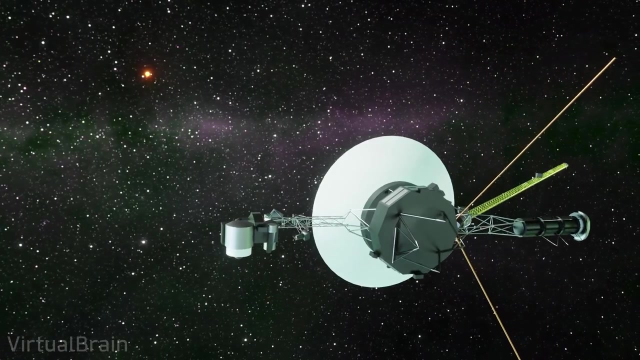 that it would be impossible to generate the energy needed to operate them using photovoltaic panels And, at the same time, due to the long mission duration, the use of fuels or chemical cells was not feasible either. Because of these limitations imposed by the context of use the radioisotope thermovalve. 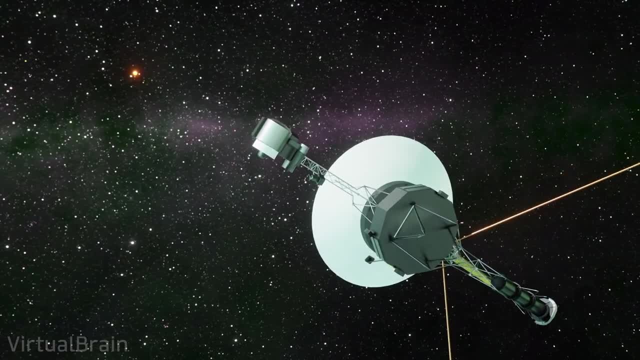 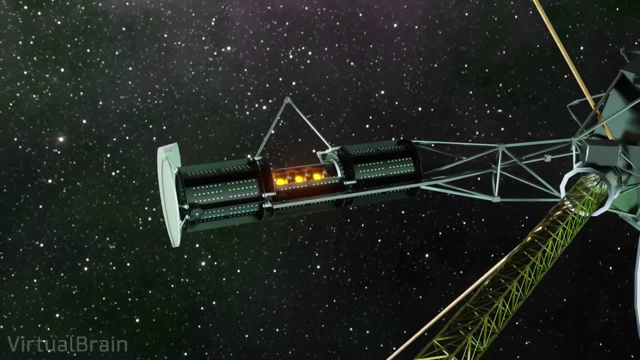 or thermoelectric generator was the only viable option to keep the probes running. The operation of this type of generator can be separated into two parts, as its name indicates: On the one hand, the use of a radioisotope and, on the other hand, the generation of electricity. 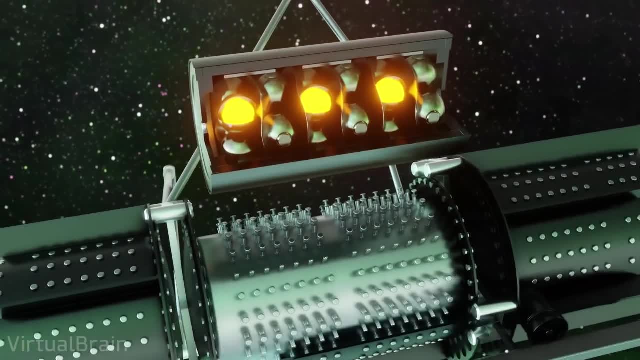 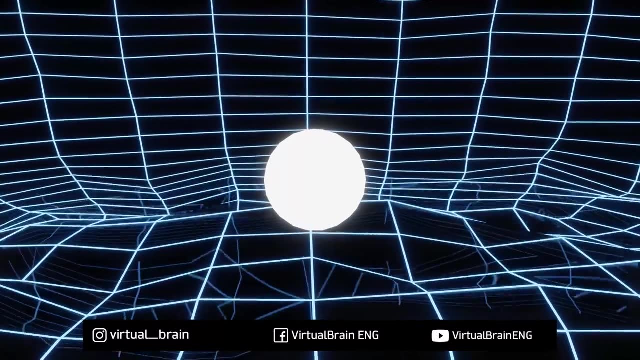 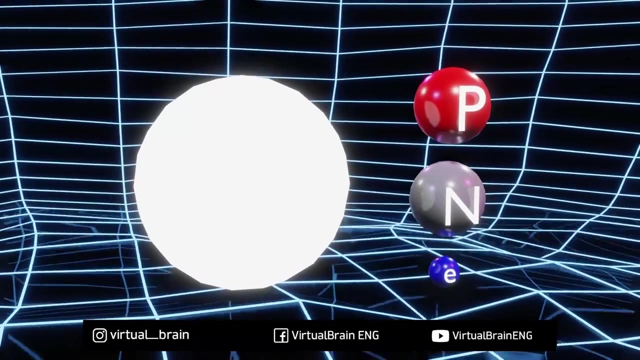 through thermoelectric effects. To understand what a radioisotope is, we must first understand how the elements are composed. In an extremely simplified way, we can say that an atom has three different elements. There are different types of particles: protons, neutrons and electrons. the number of protons? 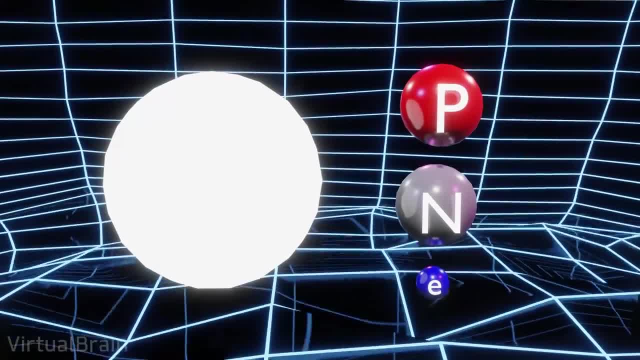 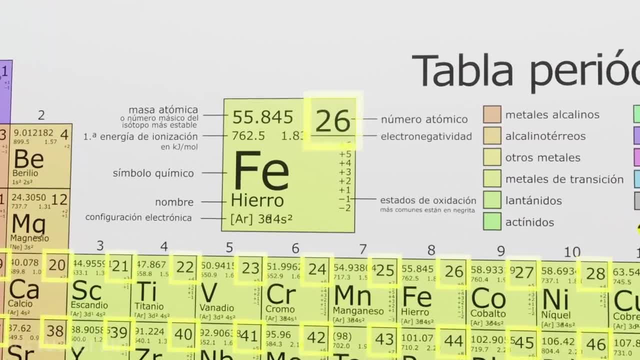 being that determines which element it is exactly. In fact, if we look at the periodic table, we will notice that in one of the corners there is a series of numbers that follow an order. This is known as the atomic number and corresponds precisely to the number of protons in the 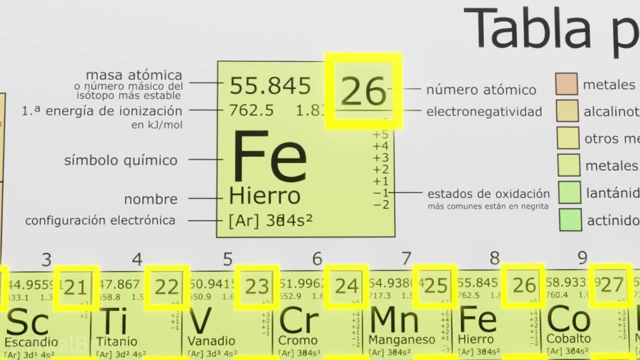 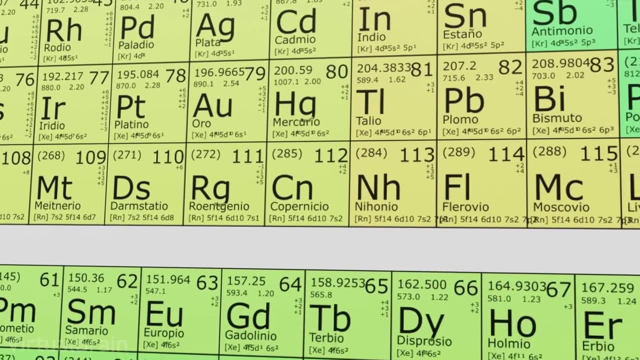 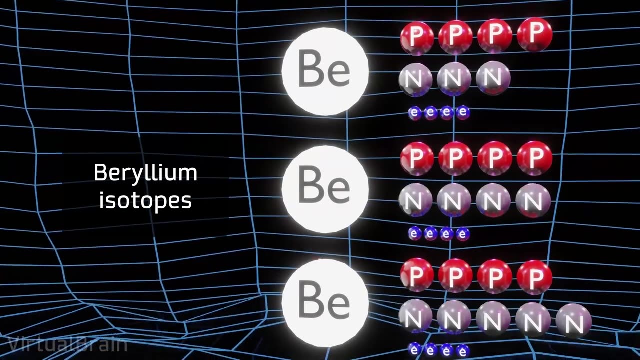 element. In other words, if the number of protons changes, the element changes. However, Both the number of electrons and neutrons in an atom can change without it becoming a different element. Considering this, the isotopes of an element simply correspond to a series of atoms with. 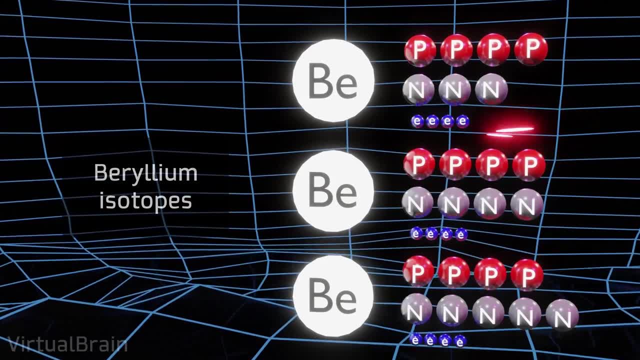 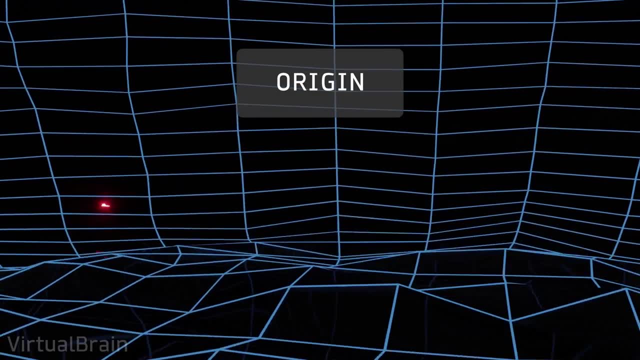 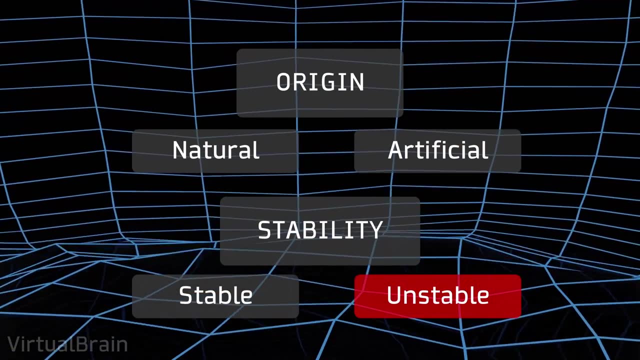 the same number of protons, but with different numbers of neutrons. But that's not all. we can also categorize isotopes on the basis of two criteria: First, whether they are naturally or artificially produced, And second, whether the isotopes are stable or unstable. 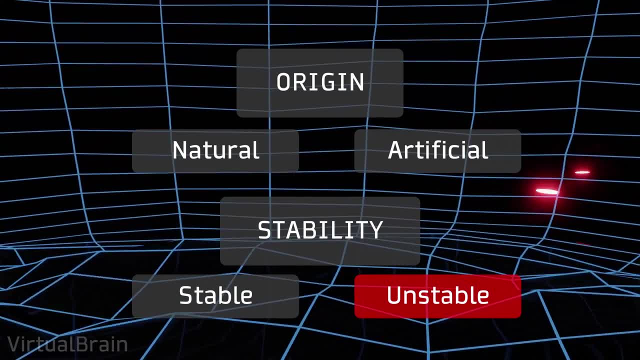 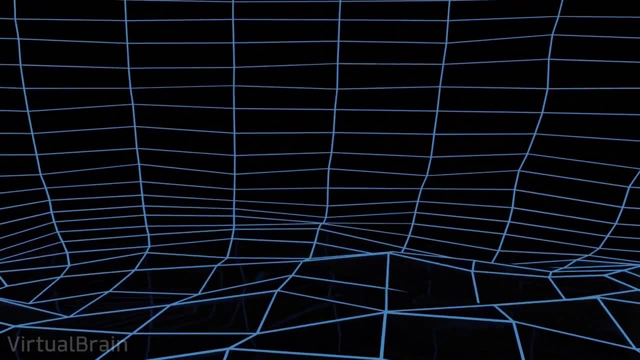 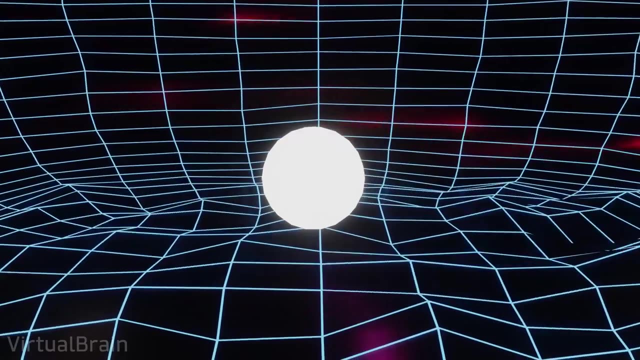 So let's start with the isotopes. The latter category is the one that interests us, since an unstable isotope is what is known as a radioisotope or radioactive isotope. This particular type of isotope, as its name implies, is incapable of maintaining its composition. 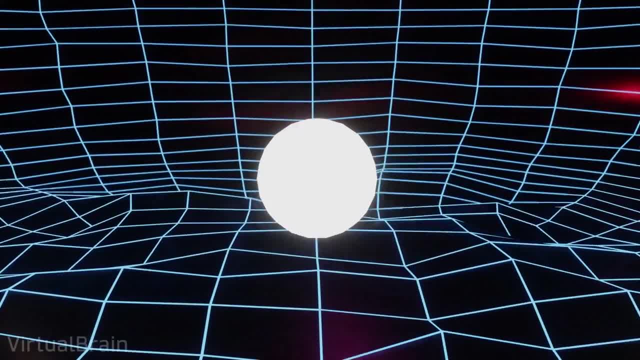 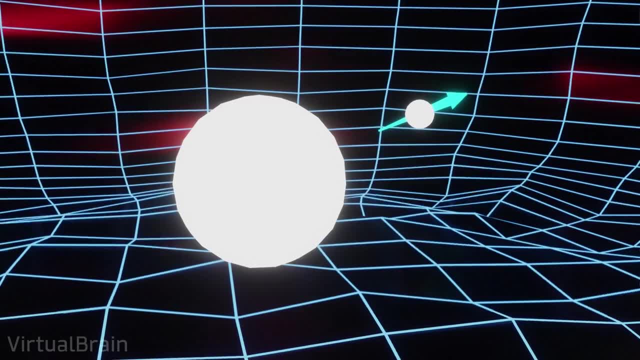 because it possesses an excess of nuclear energy. The way for it to become stable again is to eliminate the excess energy, which is done through the emission of different types of highly energetic particles, a process that is also known as radioisotope. This process is also known as radioactive decay or radioactive disintegration. 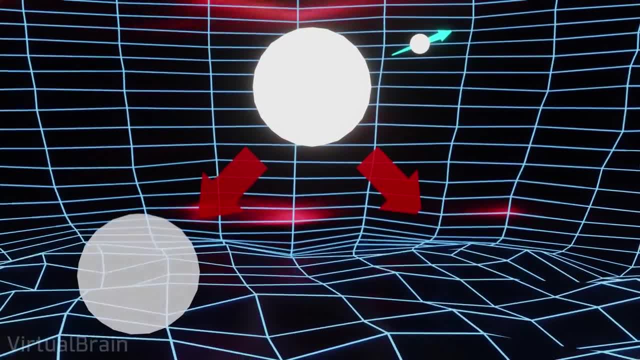 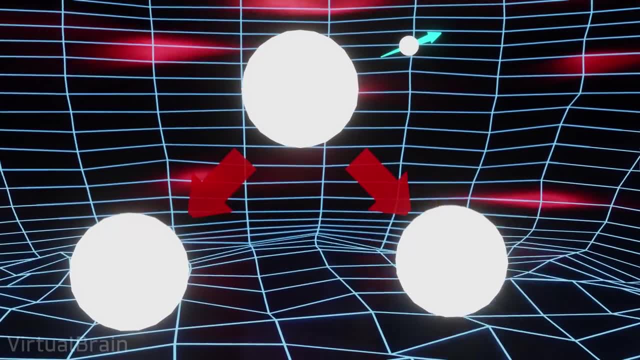 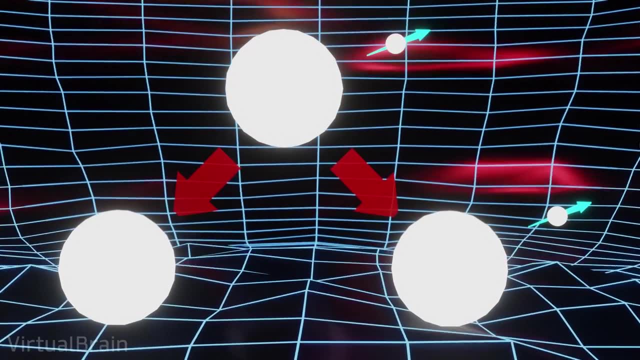 When this process occurs, there are two possible outcomes: The unstable isotope can become a stable isotope or it can become another unstable isotope, continuing the cycle until it becomes a stable isotope. Given this behavior, no unstable isotope will emit radiation indefinitely, although of 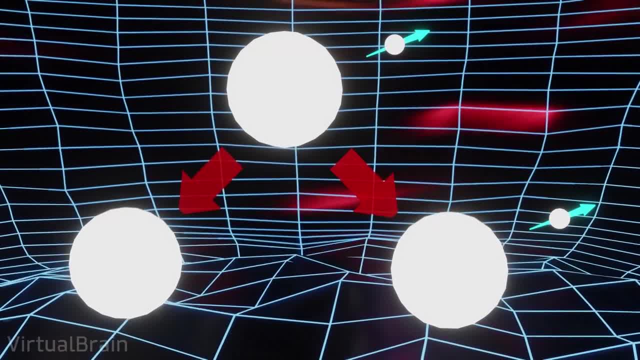 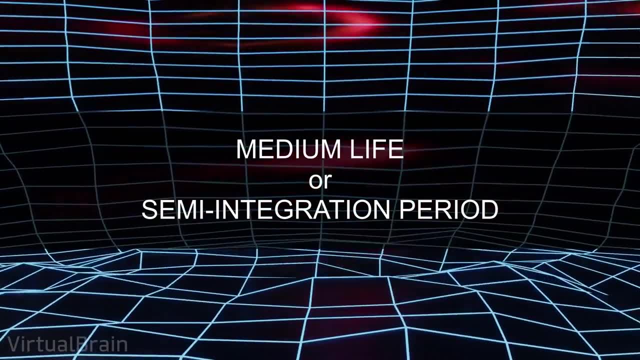 course, the rate of radioactive decay can vary greatly from one isotope to another. The most common way to measure the speed of decay is by calculating the median life, or half-life of the particles, which corresponds to the required time for half the nuclei of 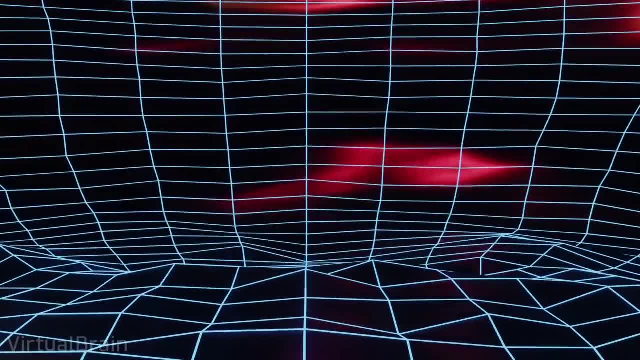 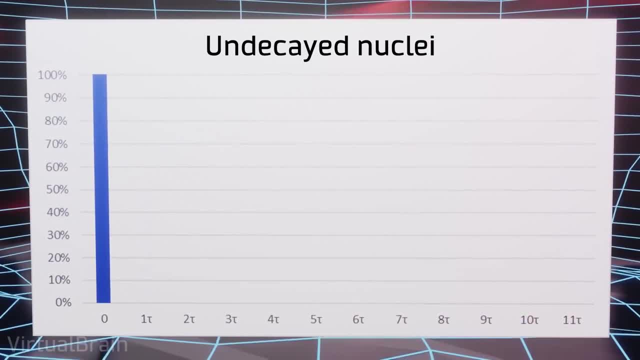 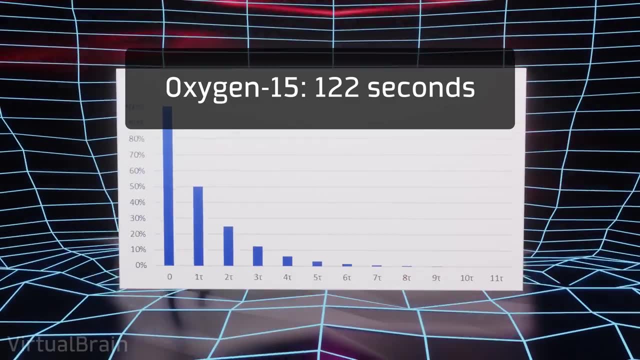 an initial sample of radioisotopes to decay, That is, if at zero time we have 100% of the nuclei without disintegration. when this period passes, there will be 50%, then 25%, then 12.5%, and so on. 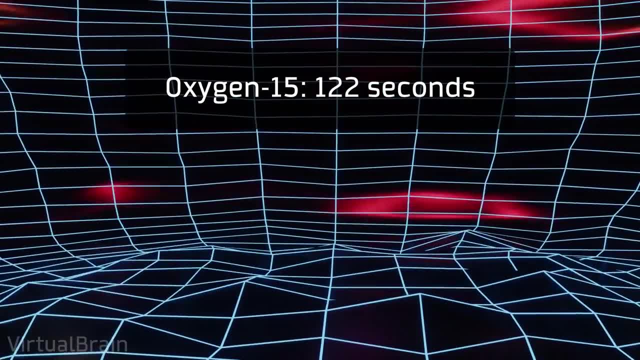 For isotopes such as oxygen-15,. radioisotopes will have a time of 50% and then 25%, then 12.5% and so on, Where 15 represents the sum of neutrons and protons of the atom. this period is just 122. 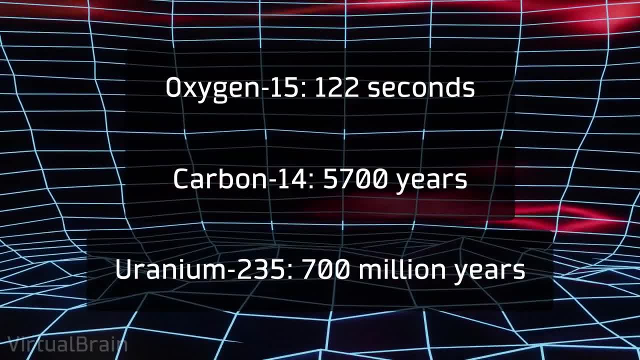 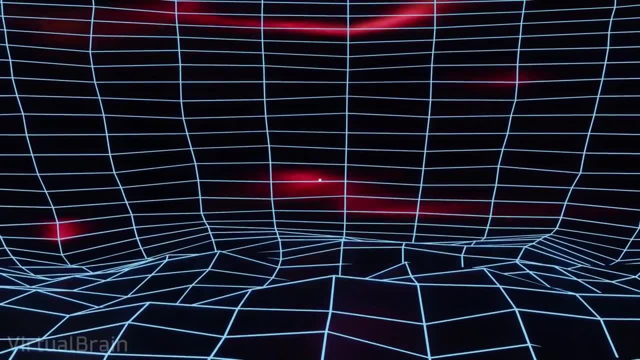 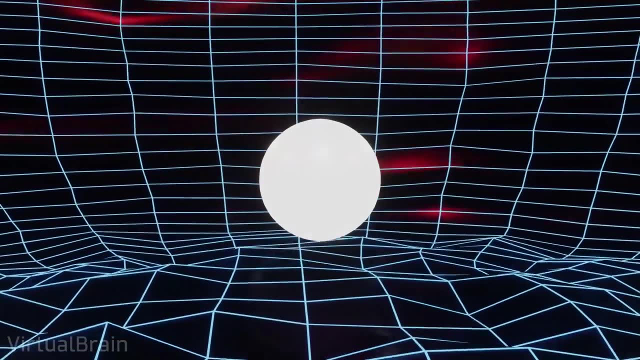 seconds For carbon-14, 5.700 years and for uranium-235, some not at all insignificant- 700 million years. But now back to the main topic. of all the existing radioactive isotopes, One of the most used in thermoelectric generators is plutonium-238, with a half-life of 87 years. 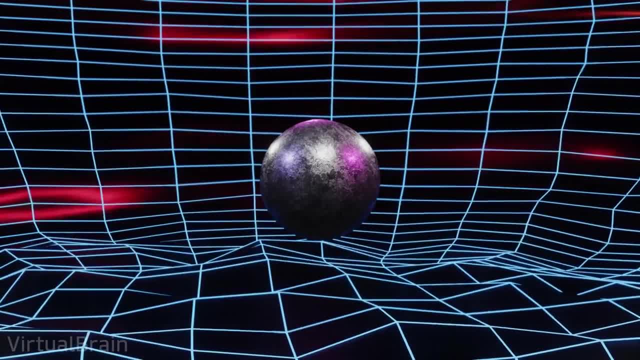 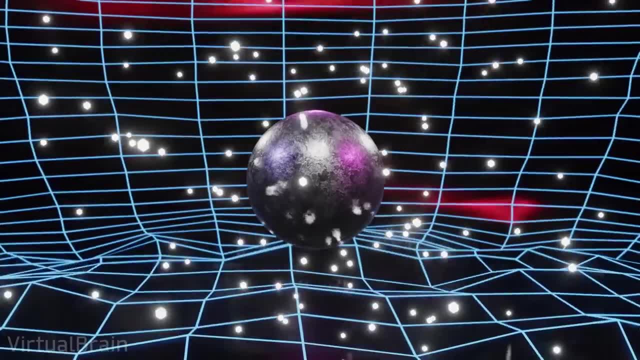 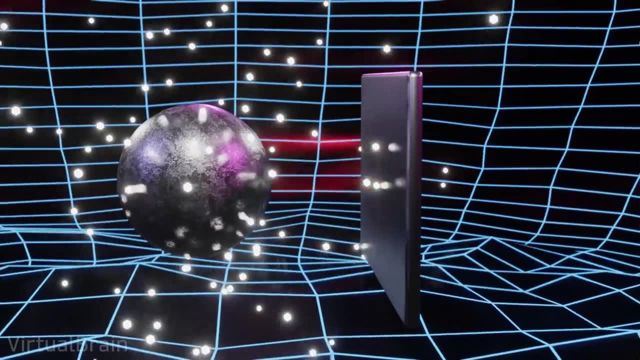 This is the most used isotope in thermoelectric generators, But even more important than that, this particular isotope is used because it disintegrates emitting alpha particles which have a high mass and therefore interact with other atoms, being easily stopped on collision with them. 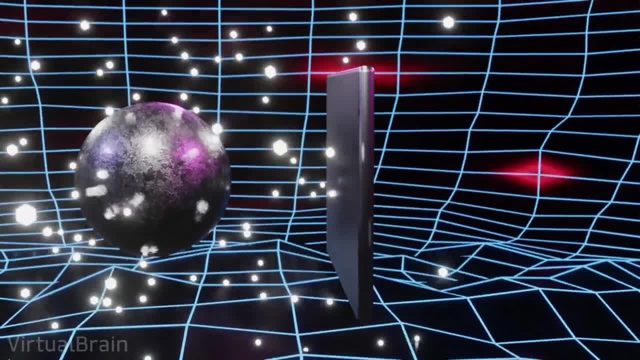 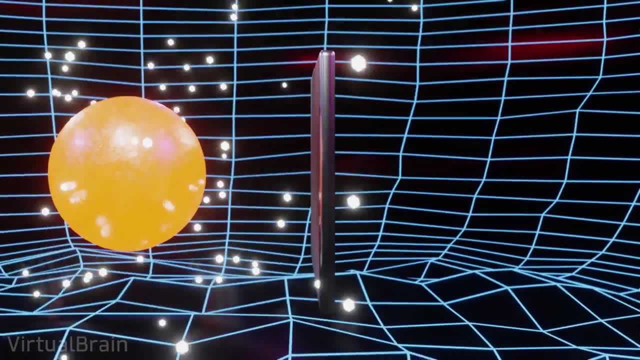 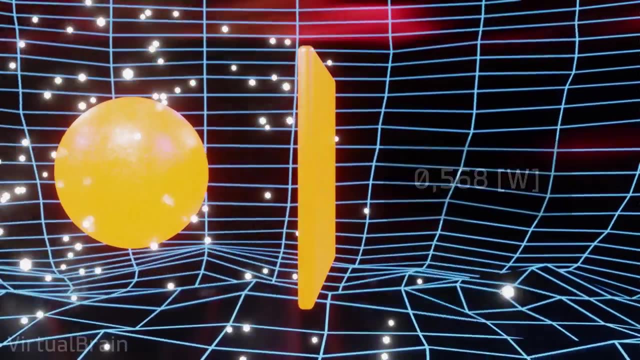 Which, in practical terms, means that if we have a piece of plutonium-238,, the kinetic energy of the alpha particles will be converted into heat upon collision either with itself or with other surrounding elements, Generating 0.568 watts per second in the form of heat per gram of this element all. 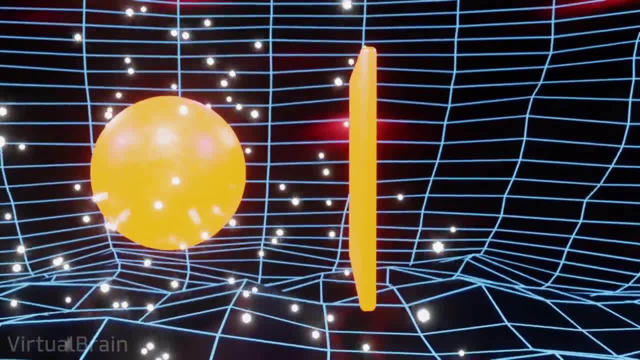 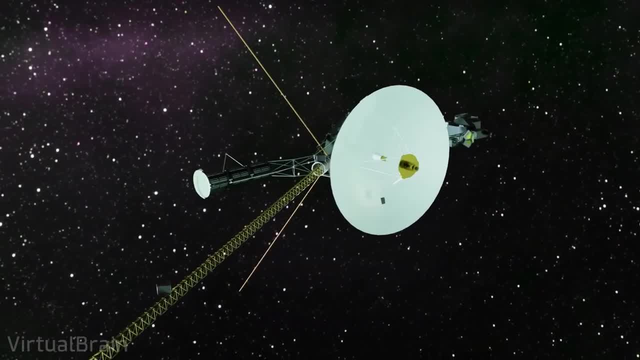 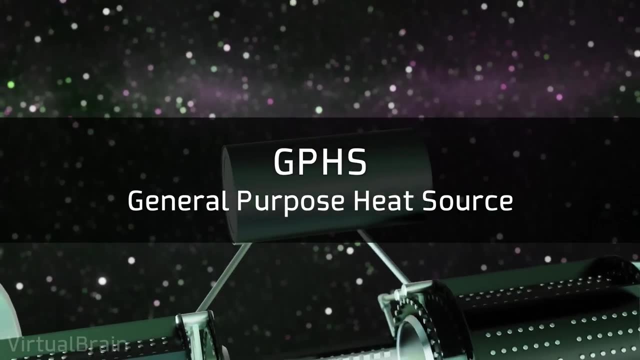 this completely spontaneously, without the need to provide an initial energy, a chemical reagent or anything like that. Understanding this, if we analyze a radioisotope thermoelectric generator from the inside, its heart is a series of elements known as GpHs or general purpose heat source, which 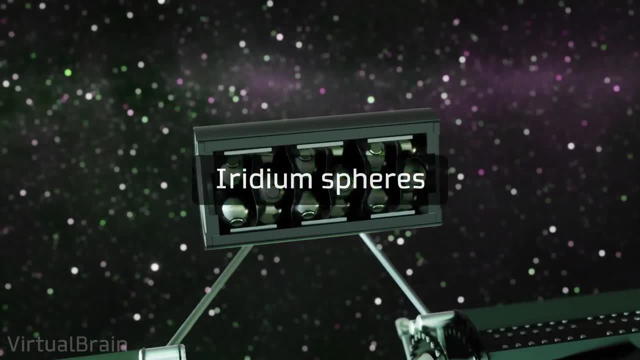 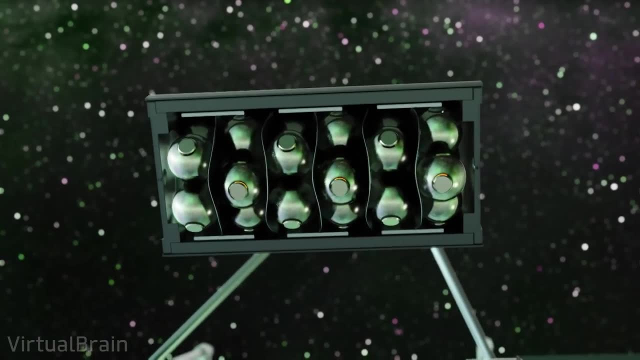 in the particular case of the Voyager probes. In the case of the Voyager probes, GpH consists of a cylindrical container with a series of iridium spheres, a metal of high hardness, high density, high resistance to corrosion and a melting point of over 2000. 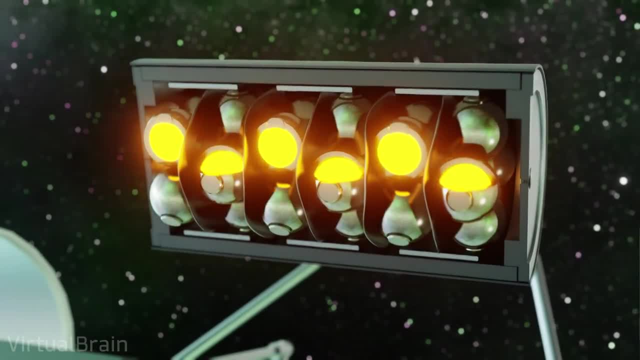 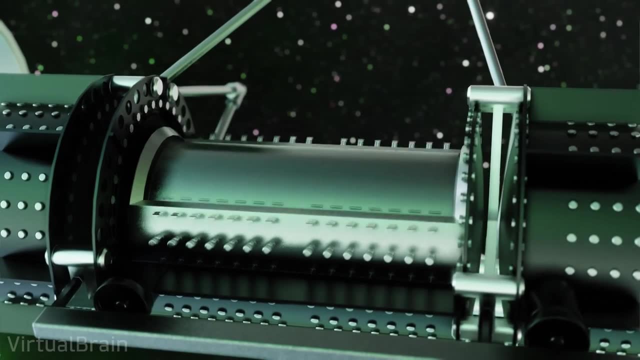 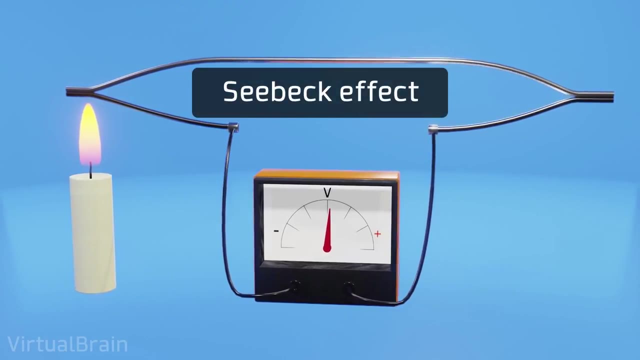 degrees Celsius. That is a perfect material to contain plutonium-238.. This general purpose heat source is then covered by a series of thermocouples which, as we saw in the previous video on thermoelectric effects, are elements that, thanks to the, 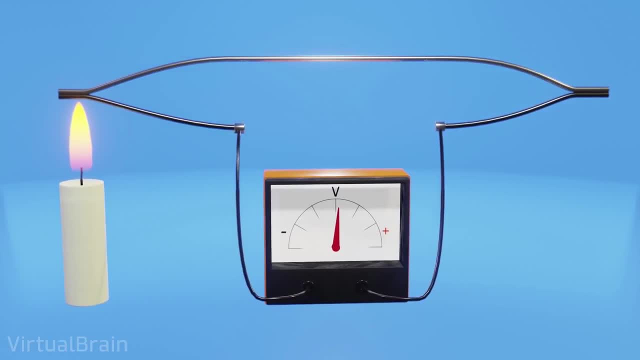 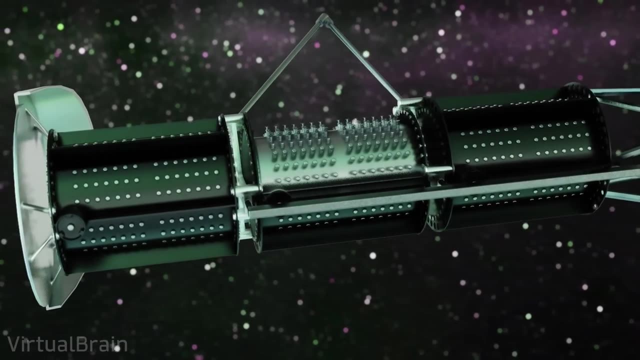 Seebeck effect. The thermocouples are able to generate a voltage when there is a temperature difference between their two junctions, And because the temperatures in space are extremely low, differences of up to 700 degrees Celsius can be generated between the inside and outside of the generator. 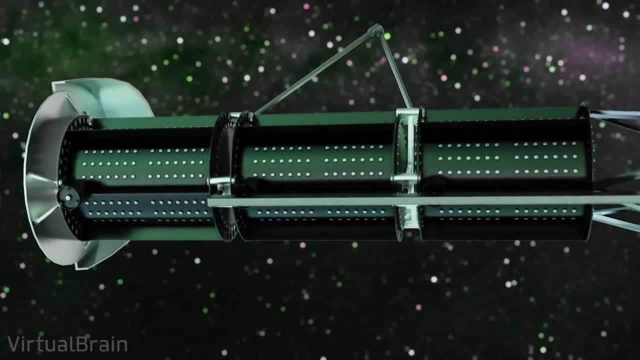 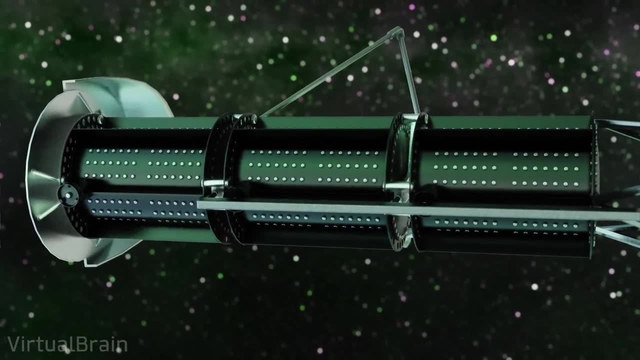 Finally, the thermocouples are covered by a final layer which serves both a structural purpose and the purpose of dissipating the heat generated inside. The Voyager probes have three radioisotope thermoelectric generators. The thermocouples are also able to generate a voltage when there is a temperature difference. 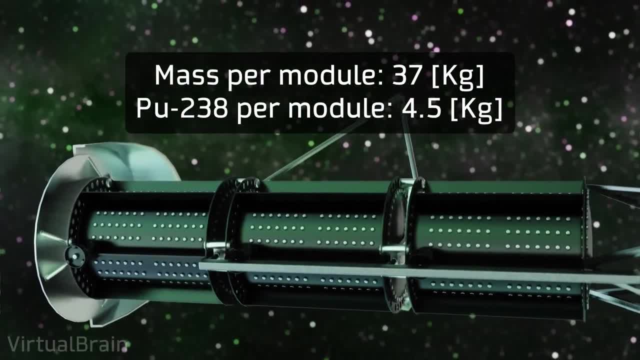 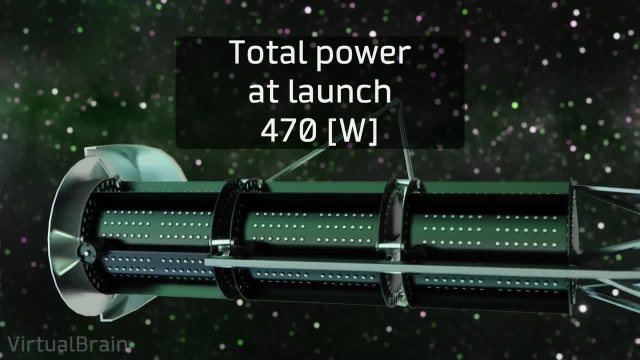 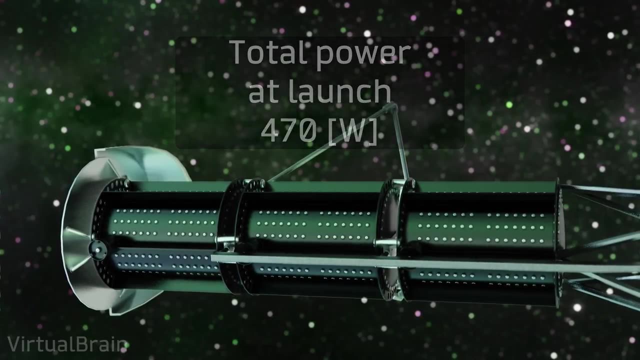 between their two junctions, Each with a mass of 37 kilograms, of which 4.5 kilograms were plutonium-238 at launch, and which together were capable of generating a power of 470 watts. Now, after taking a thousand turns, we can finally talk about why I said that these generators 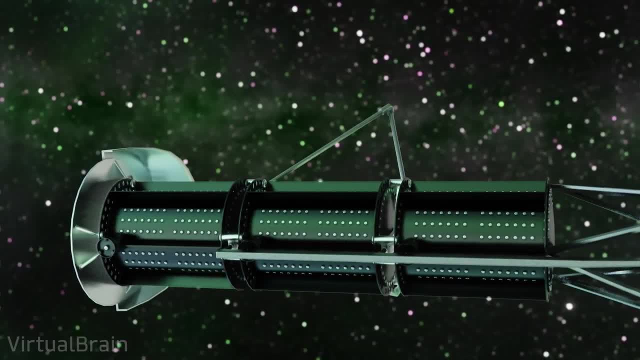 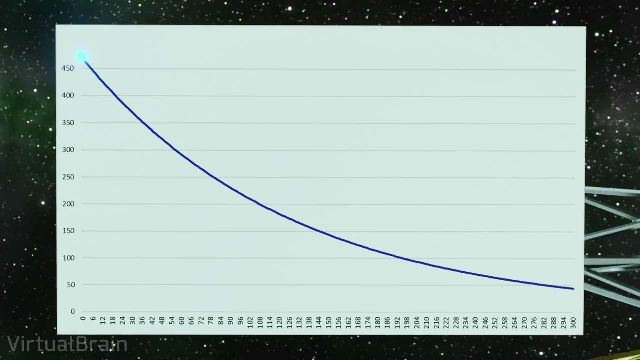 produce almost infinite power. Remember the half-life of plutonium-238? It took 87 years for only half of it to disintegrate. The thermocouples are also able to generate a voltage when there is a temperature difference between the inside and outside of the generator. 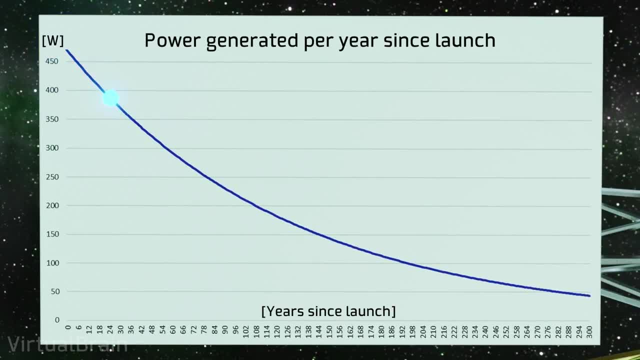 That is 87 years after its launch. theoretically, the system will still be able to generate about 235 watts In 175 years, 117 watts and so on, which is much more than we could ask of any other type of battery. 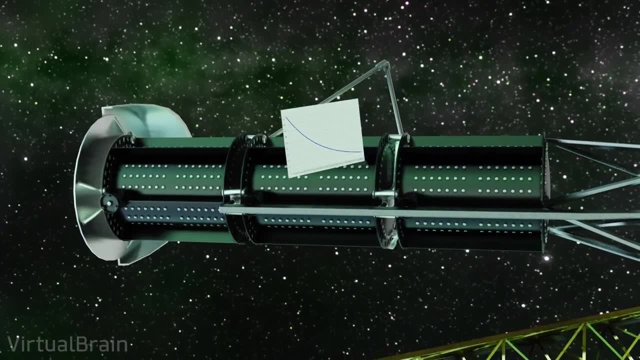 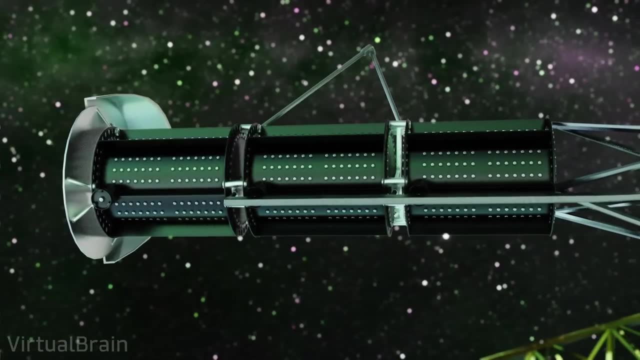 Although, of course, there are other factors that make the reality very different from the theory. for example, in the case of thermocouples, although they do not fail easily, since they do not have moving parts, their efficiency will be affected after years of use. 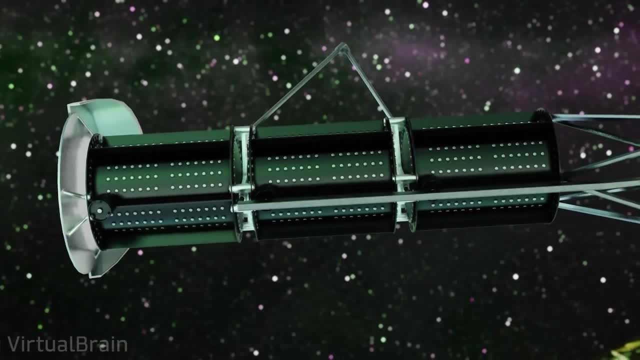 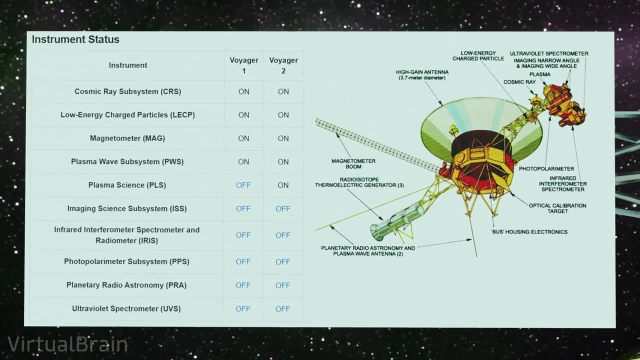 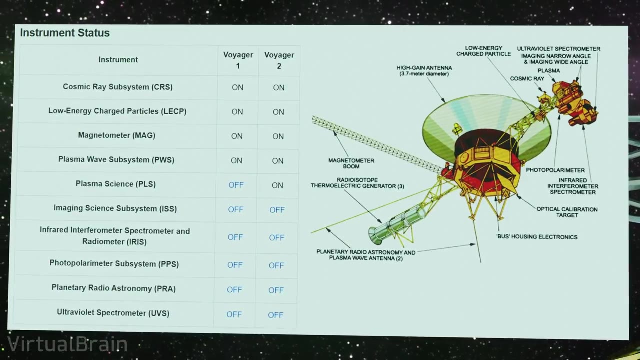 Furthermore, even if they continue to generate energy, this does not mean that it is enough to power all the probe systems. In fact, if you go to the NASA website, you will see that most of Voyager's instruments are turned off, which is probably one of the reasons why it is still able to function, even 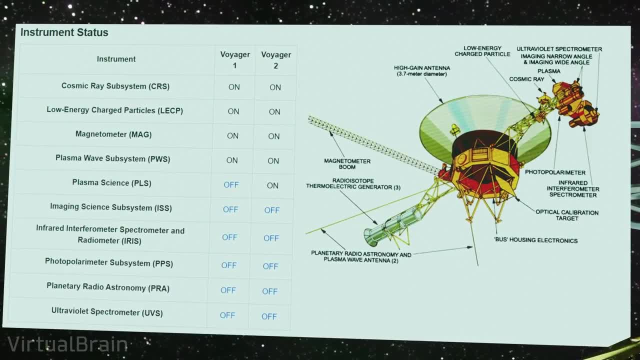 after 40 years, By which time the generators should be generating about 70% of the energy. This is probably one of the reasons why it is still able to function, even after 40 years, by which time the generators should be generating about 70% of the energy.